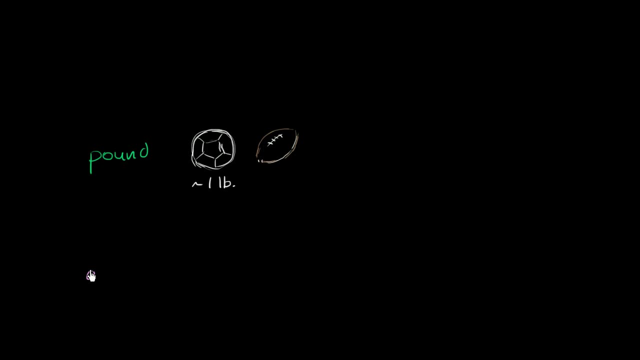 You would think about using the ounce And the relation between the ounce and the pound when we're thinking about weight. is that one pound? let me write this: one pound is equal to 16 ounces Is equal to 16 ounces, Or another way of thinking about it. 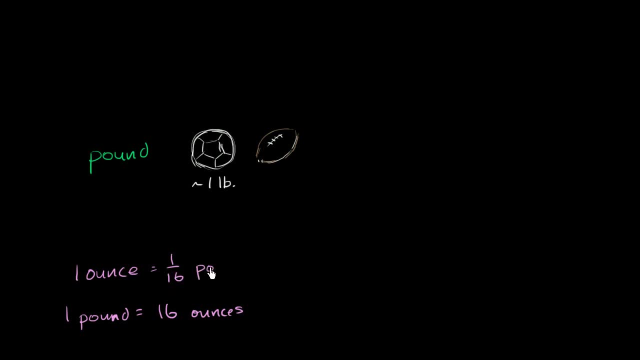 is that a one ounce is equal to 1, 16th Of a pound, And if you want to visualize things that weigh about an ounce, you could imagine a small box of matches weigh about an ounce. So a small box of matches might weigh about an ounce. 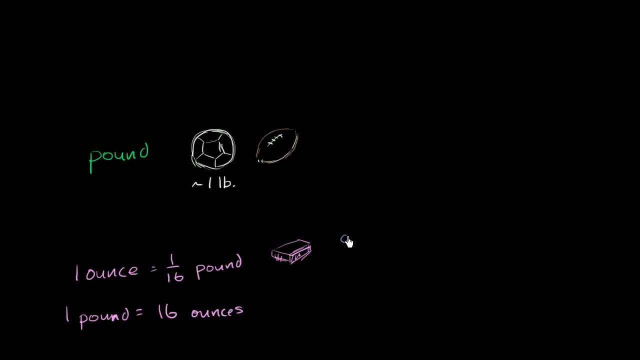 Maybe a small AA battery would weigh about an ounce, But that gives you a sense of it. So if you were to take 16 of these together, they would be about the weight of a soccer ball. 16 of these things together, they would be about the weight. 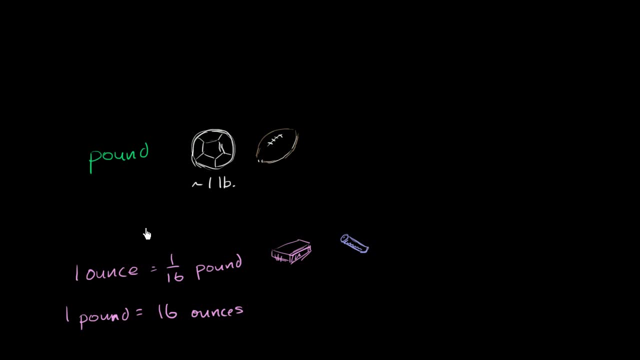 of a soccer ball or a football. Now, if we want to think about weights that are larger than a pound, then we would go to the ton, And a ton is equal to one. ton is equal to 2,000 pounds. 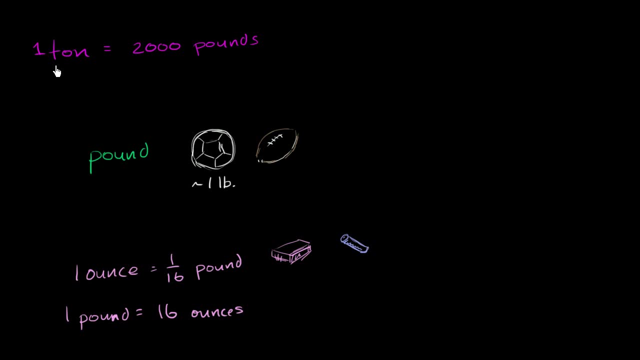 And you have to be a little bit careful with the ton. We're talking about the US customary units And this is where we're talking about 2,000 pounds, But when we're talking on a more international level, this is sometimes called the short ton. 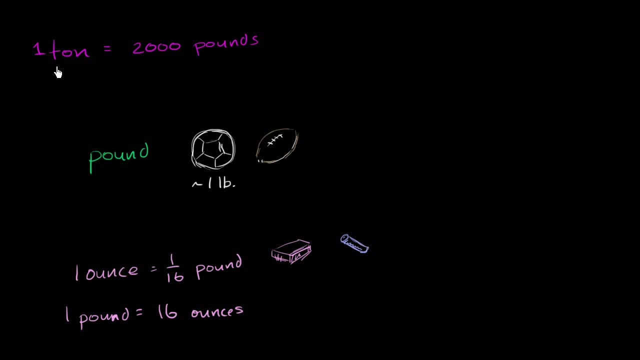 There's also a long ton. There's also the metric ton, But here we're talking about US customary units, which is the short ton. So one ton is 2,000 pounds, And to get a sense of something that weighs 2,000 pounds, or to get a sense of what 2,000 pounds is like or what might be measured in tons. a car is a good example: Your average mid-sized sedan, Your average mid-sized sedan, would weigh about a little under to a little over 2 tons. So a little under to a little over 4,000 pounds. If we're talking about a small van or minivans or vans or trucks, we're thinking it's going to be larger than 2 tons, And if you think about smaller cars, 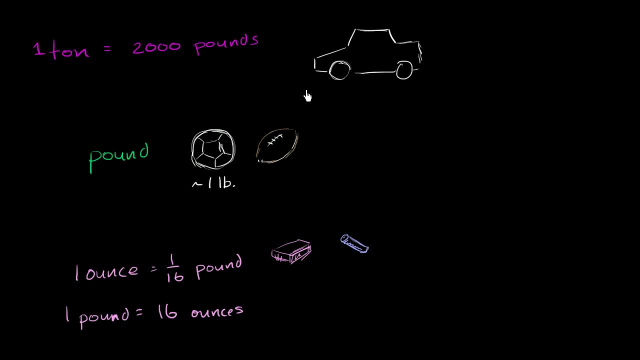 you're thinking it's going to be probably around 3,000 pounds. It's going to be less than 2 tons. So a car is going to be a product. It's going to be approximately 2 tons. So hopefully that gives you a sense. 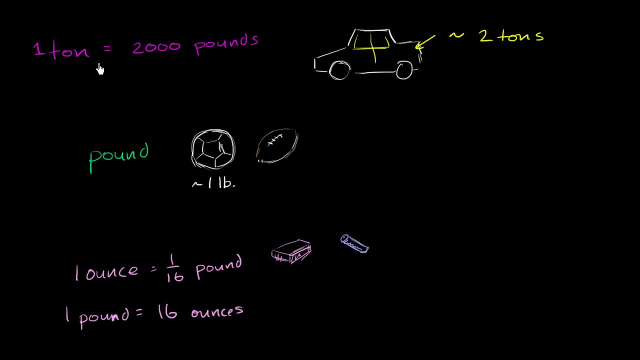 of what units you would use in the US customary system for different scales of weights.